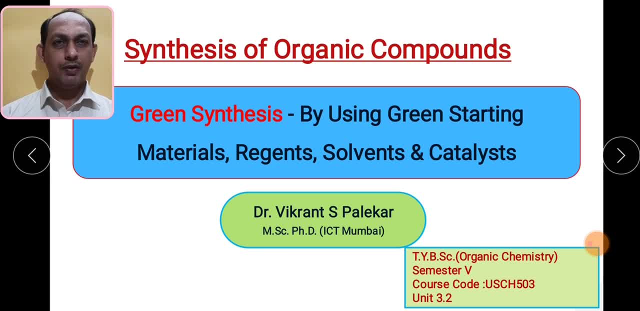 particular topic, we have seen different terminologies, such as what is ideal organic synthesis, what are the different types of organic synthesis, then managed reaction and beginning reaction. in the topic of multi-component reactions, Then we have seen a very important topic which is quite emerging one in the field of chemistry, that is, green chemistry and principles related. 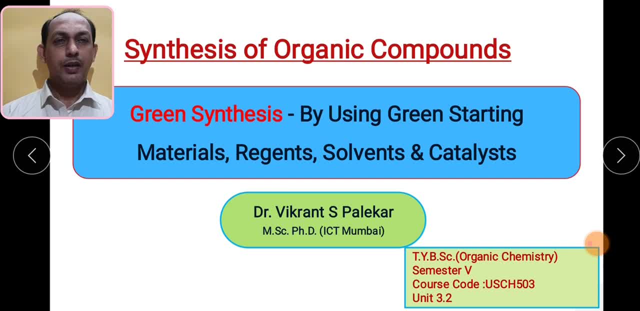 with the green chemistry, Then right now we are also in the position to know the terminologies such as: what is percentage increase yield, theoretical yield, practical yield, atom economy and E factor. So such as these things we have already covered in this particular topic. 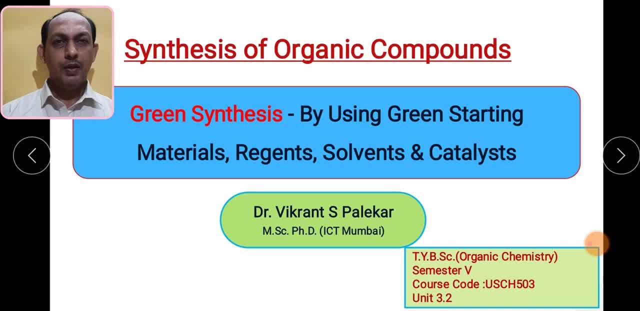 So from this particular session we are going to see green synthesis by using green starting material, reagents, solvents and catalysts. As we know, the traditional layout of the any organic reaction, where any particular substrate reacts with the reagent and it forms product and byproduct. 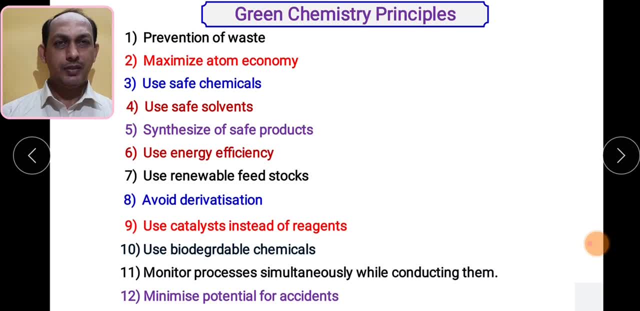 As we have already seen, the principles of green chemistry. So it is basically related with the formation of waste or hazardous waste material which are formed inside the any reactions. So In this particular four important components of the any reaction, that is substrate, that is also we called as a raw material, then reagent and product. 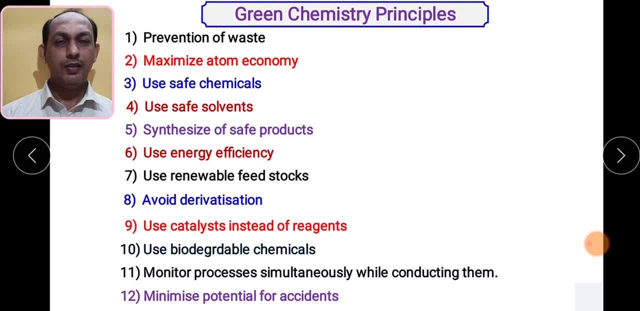 And also one thing comes in the reaction, that is catalyst. See all these things, three things must be renewable, or must be green in that perspective, So that Whatever the waste form Will be minimized. So these are all twelve principles of green chemistry. 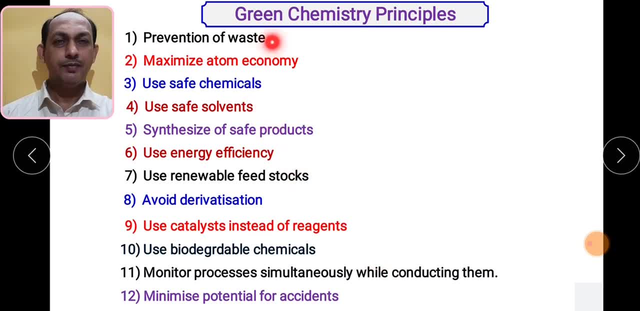 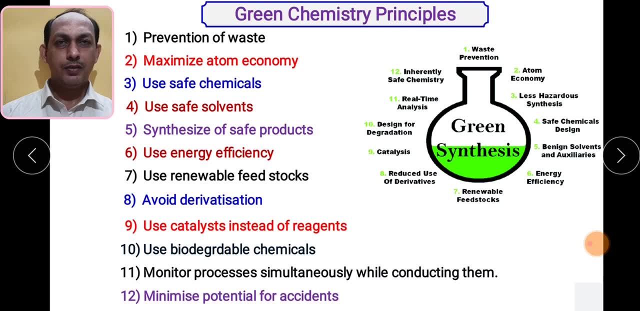 So it basically talks about waste prevention. So in order to have the green synthesis, we must have four components which are very important: Whatever the raw material we are going to use, that must be green in the perspective of renewable feedstock. Then, whatever the reagent we are going to use, 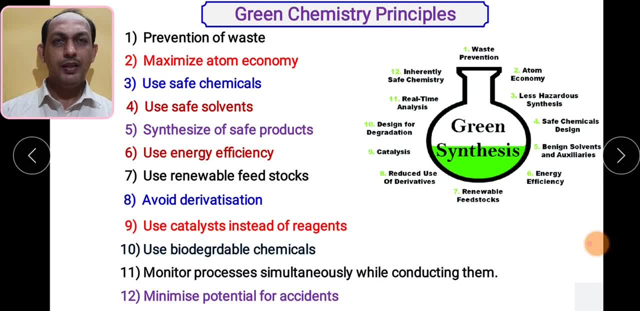 That must be green. Then catalyst it also be a green in the form of, then whatever the product we are going to get, that also be green. So if you carry out all these four components in effective manner, that particular synthesis will be green synthesis. Now we are going to see the basic things related with the green synthesis. 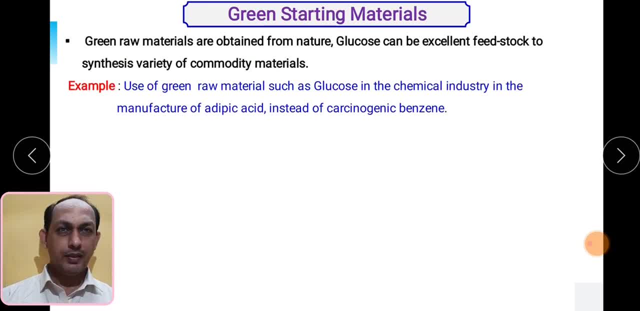 So first thing we must taken care of, that is starting matter. whatever the starting material we are going to use in the organic synthesis, that must be green. green in the form of that particular raw material must be obtained from the nature. that must be, i think, renewable and biodegradable inside the 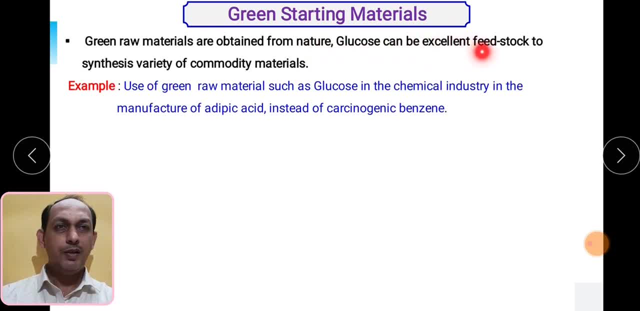 nature. so, as we know that glucose is one of the very important feedstock that can also be used for the synthesis of variety of commodity chemicals. if we use such a raw material, for example, for the synthesis of adipic acid, as we know, the traditional method for the synthesis 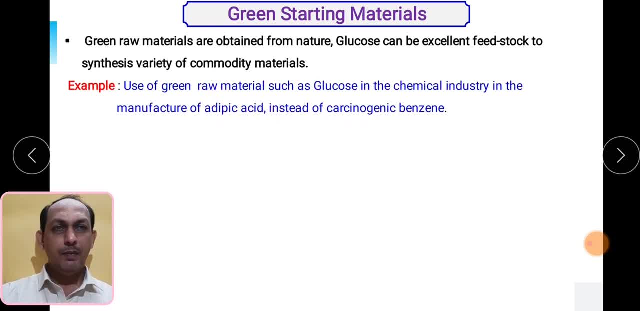 of adipic acid is from the benzene and as we know, that benzene is carcinogenic material. so if you start that particular synthesis with the help of glucose, then that will be a very good green starting material, as we know that conversion of glucose into adipic acid can be carried out effectively by using a biochemical. 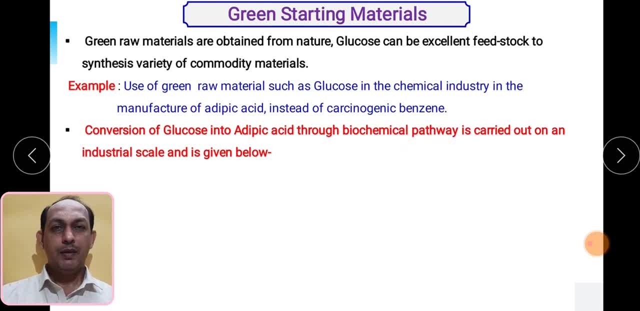 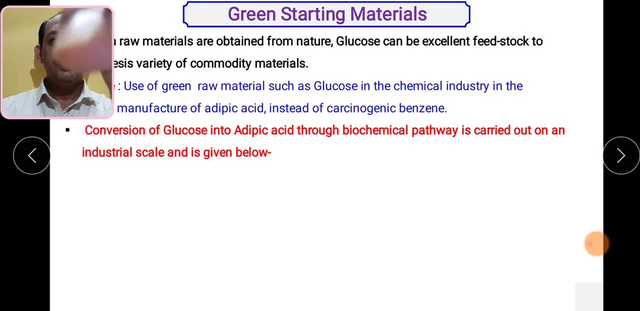 pathway. biochemical pathway means this particular reaction can be catalyzed by using enzymes and at industrial level also, this particular synthesis is carrying out effectively. let us see that particular reaction. first, you have to start with the glucose. as we know what is the formula- c6, h12, o6, so it is very easily available feedstock. 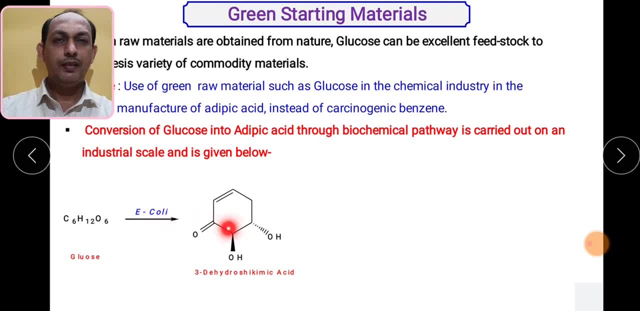 we carry out the reaction with the help of ecoli, then this particular compound will get converted into cyclic compound, and that is nothing but 3-dehydroemosicimic acid. so this is a 3-dehydroemic acid form, first through biochemical pathway, then, again with the help of ecoli, we can open this. 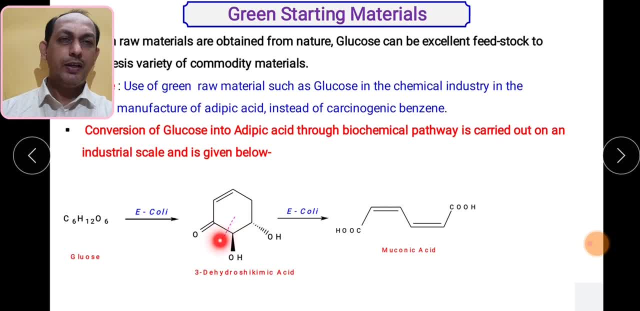 particular chain and this particular carbon carbon bond undergo breakdown and then to another part of the and you get the formation of open chain compound that is being called as a muconic acid. so it will have at both the side coh groups. then this muconic acid, with the help of hydrogenating reagent such 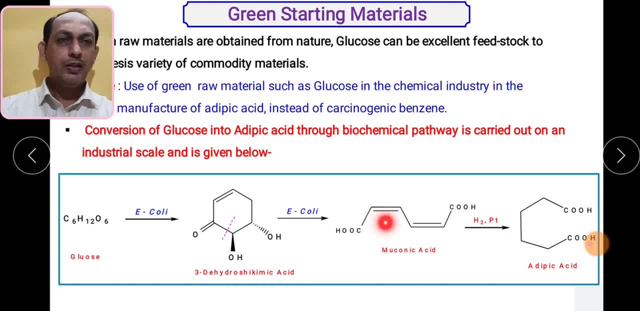 as h2pt, it undergo reduction of this carbon carbon double bond and you get the formation of adipic acid. adipic acid is six carbon compound and, as we know that adipic acid is very effectively used as a raw material in the manufacture of nylon 66 fibers, so it is very advantageous to 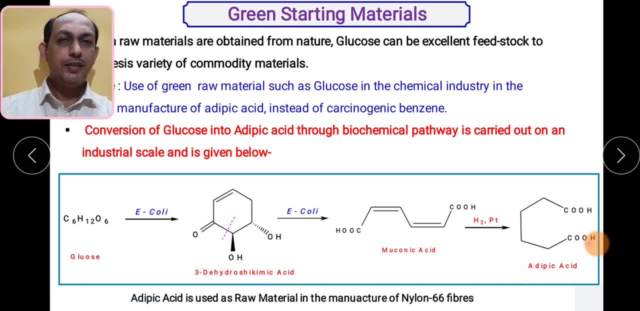 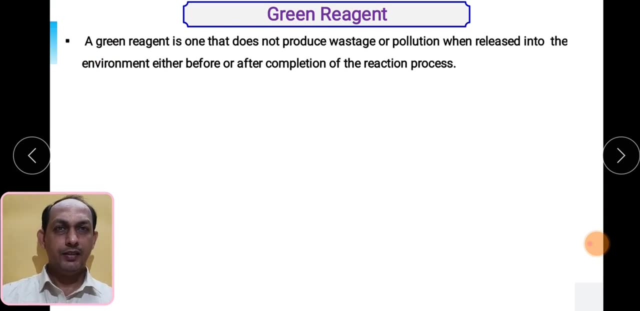 use this particular synthesis of adipic acid from glucose, so that particular synthesis will come under the principle of green chemistry by using green starting material. then, second aspect: we are going to see that is a reagent, the reagent water you are going to use in the synthesis. that must 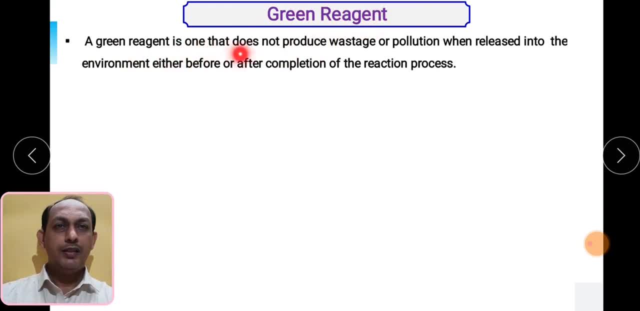 be green. so green reagent is one that does not produce waste or pollutant when released into the environment, either before or after completion of the reaction process. reagent water we are going to use that should not produce effluent or waste inside the environment after the reaction is over. 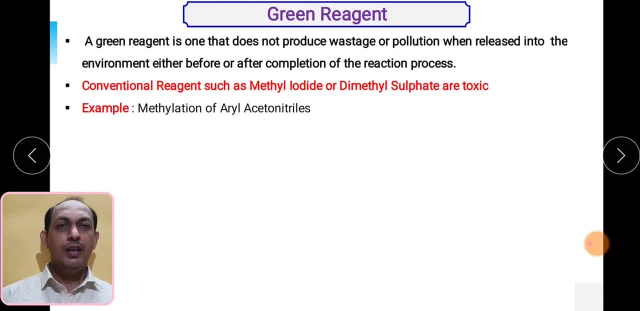 so let us see what is the reagent. as we know that conventional reagent for carrying out methylation, for introduction of CH3 groups, we generally use methyl iodide or dimethyl sulfate, and as we know that these are very toxic materials, so what is the alternative for that? we can go for reagents just. 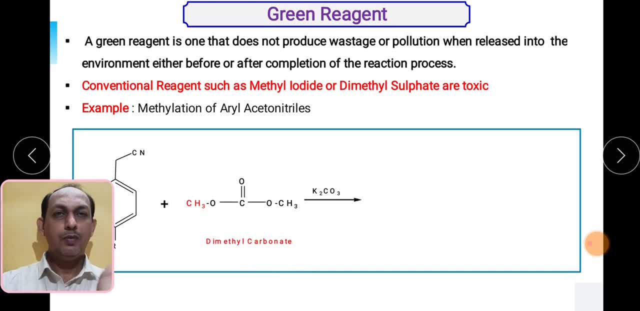 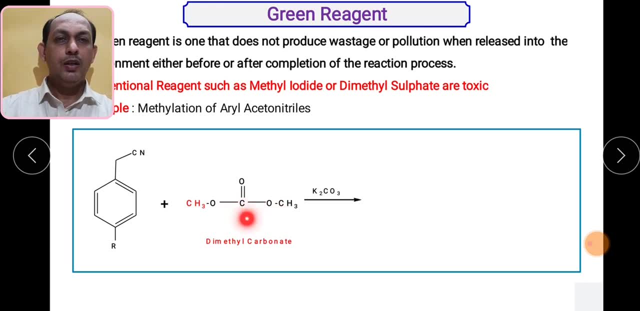 like a dimethyl carbonate. so dimethyl carbonate is the compound which is having. CH3O is flanked in between the two carbonyl groups. so if you want to carry out methylation of aryl acetonitrile, you should not use an N維 as an N alkylmic疆h reaction with a блKa of a. cry часть Gravity of methalic, Gabriel and thebuat crying you and this particle carbon. so this is a much more effective elasip Millennium belooru in the presence of pitもしu, three solvents. so what will happen? this theory is a selective methylation in at this particular carbon, so this is a ar. 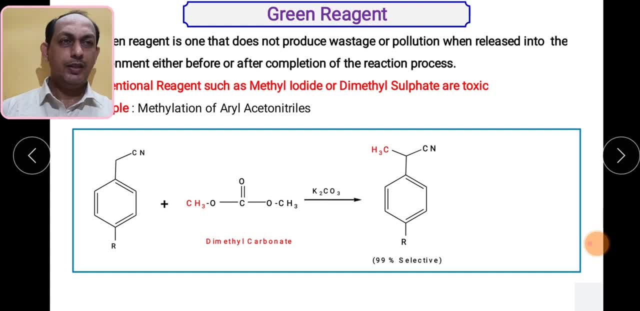 as a very green reagent which is very effectively used for the methylation of aryl acetonitrile. it can also be used for methoxycarbonation of amino group or to bring about selective methylation at active methylene groups. so it is very green reagent as the perspective point. 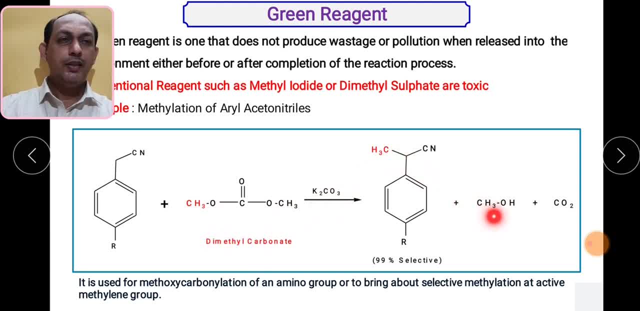 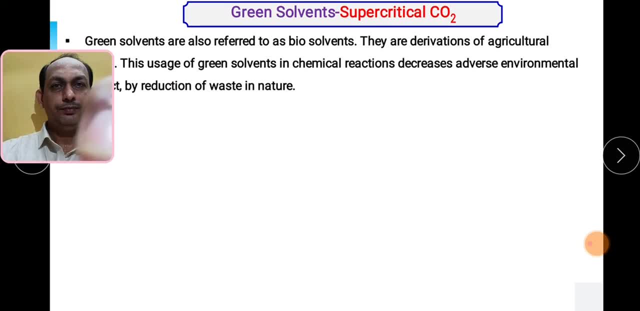 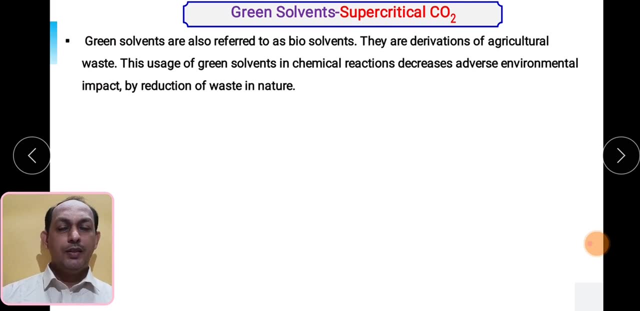 because after the methylation it get converted into ch3os and carbon dioxide, so we can say this particular reagent it quite green one. then very important aspect is the solvent. as we know, solvent is the one which used to dissolve substrate and reagent, so it forms. 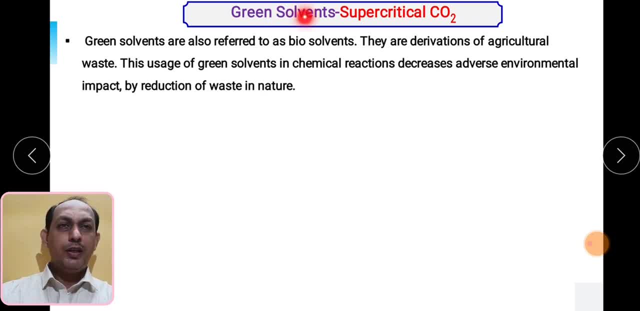 basically homogenous mixture, so solvent must be also green- green in the terms of its hazard factors. so green solvents are also referred as biosolvents because they are derived from agriculture. so it is a very green reagent. so we can say this particular reagent it quite 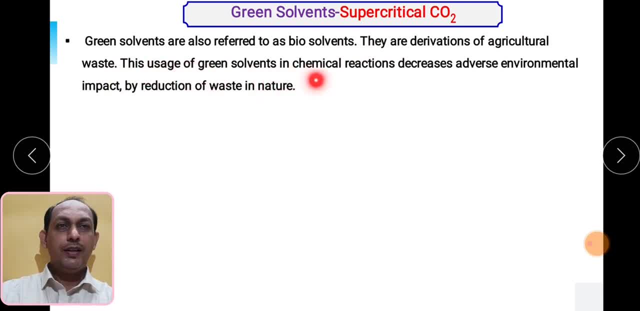 green one. then, very important aspect is the solvent. as we know, solvent is the one which used to dissolve substrate and Homogeneously produce its own Plasticержre frame. whatever the solvent we use, landlord- and it has- it has a very adverse effect on the environment, so it generally accumulates the role of waste formation. if 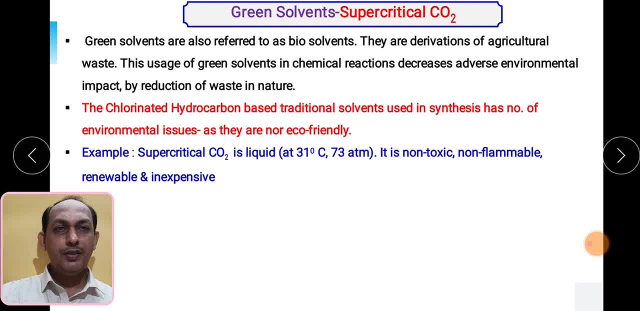 solvents being used. generally, chlorinated hydrocarbon solvents are traditionally used and we know that the solvents such as chloroform, tetrachloromethane, dimethyl chloride. so these are the solvents basically used, but as we know that this chlorinated hydrocarbons have a lot of 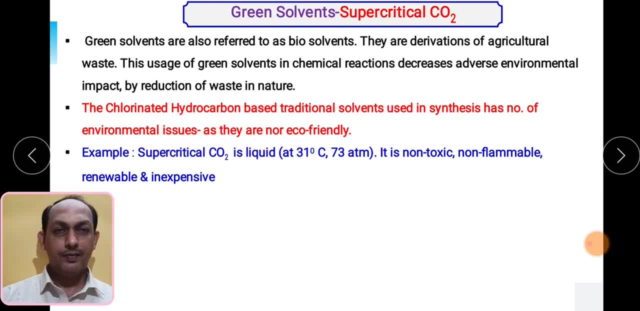 environmental issues as they are not eco-friendly, so they are having a lot of hazards issues with their uses. so if you go for such a green solvent such as supercritical carbon dioxide, which is liquid and basic property is that it is not toxic, not flammable, renewable and 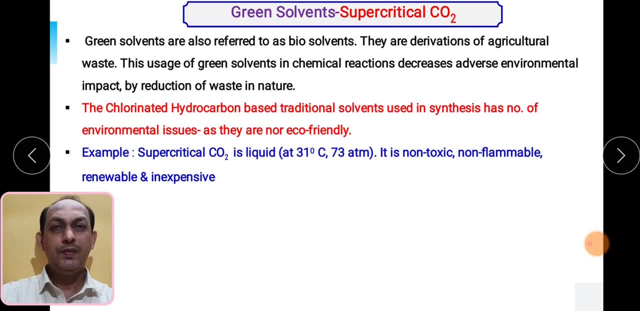 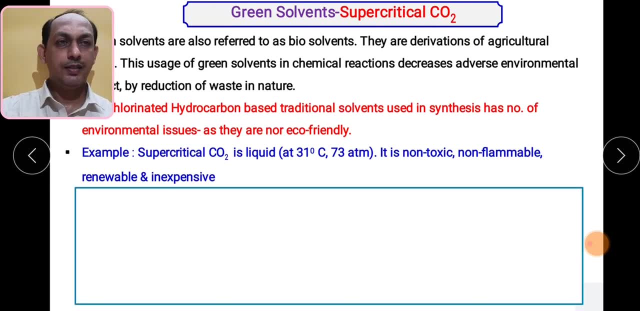 inexpensive also, so supercritical carbon dioxide is very good choice as a green solvent. so where can we use this particular solvent? let us see if you want to carry out the bromination in the toluene, so we will use the reagent n-bromo succinamide, and this is being used very. 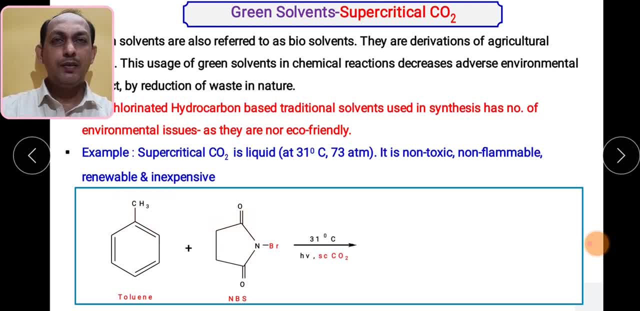 selective bromination. so in this case the bromination will take place in the side chain. if you use, for this particular reaction, supercritical carbon dioxide in presence of photochemical pathway, so what will happen? you will get the selective bromination that is ch2br. so you will get the formation of benzyl bromide with 100 percent selectivity. 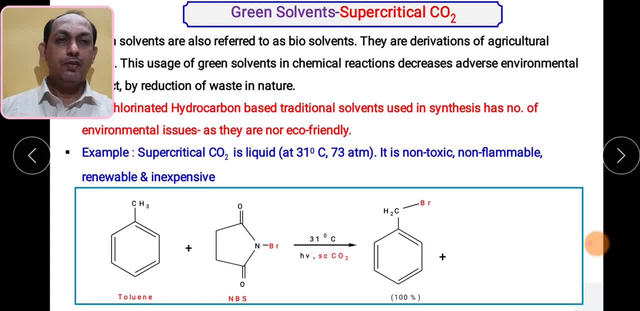 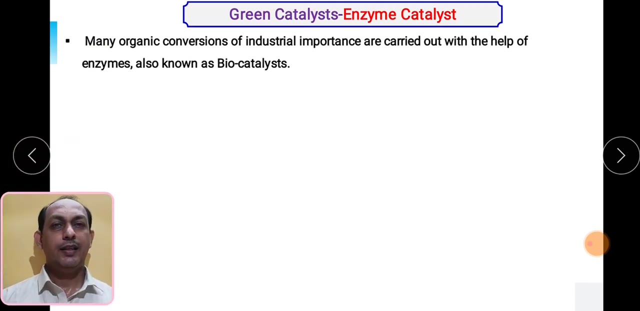 so this particular reaction can be very effectively carried out by using supercritical carbon dioxide with the formation of, again, thalamide. so here we can use the supercritical carbon dioxide. nowadays it is being very conventionally used for the carrying out different organic synthesis. then next one, catalyst. as we know, that catalyst the nowadays a very important entity for carrying. 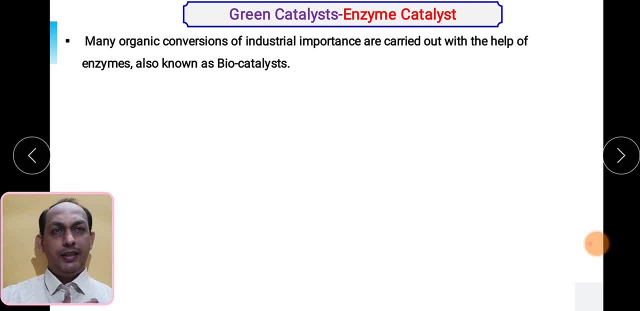 out any organic synthesis. so if we go for green catalyst, such as enzyme catalyst, that particular synthesis will be very effective one by using green catalyst. so, as we know that in at industrial level, many organic conversions are carried out with the help of enzymes, and such reactions are: 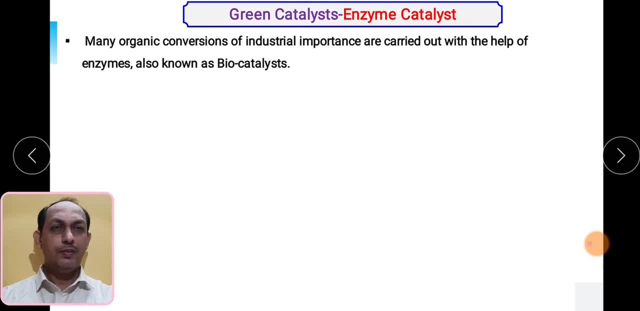 called as a bio catalyst. they use bio organism for carrying out catalyst. what are the advantages of bio catalyst? first one: it is a reaction we can carry out in aqueous medium, so we don't need any special solvents, so water can be used very effectively as a solvent. then these reactions are basically a single step, reaction only in one. 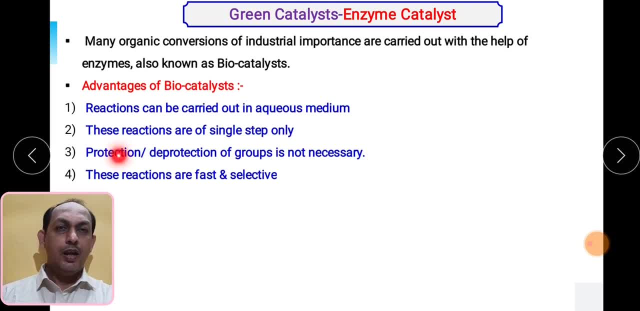 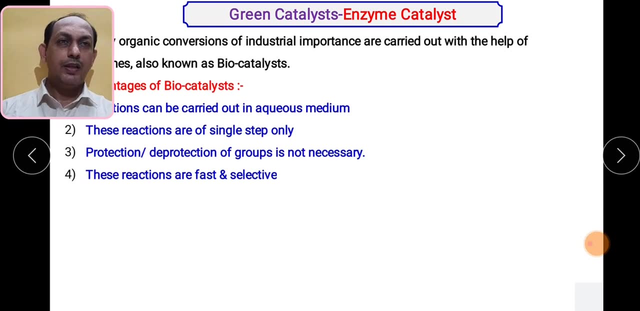 step we get the desired product. and when you use such bio catalyst, there is no derivation such as protection, deprotection of the groups need not to be carried out, and these reactions are very fast. so these are the advantages of enzyme catalyst. so where we can use the enzyme catalyst reaction, let 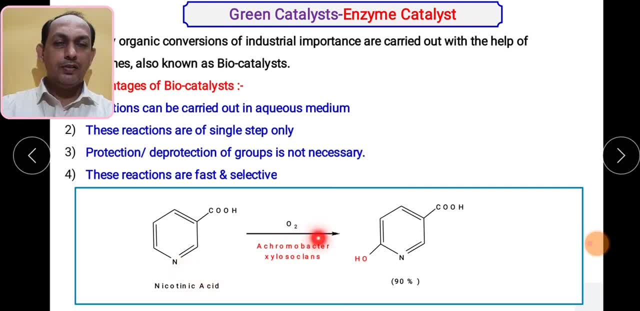 us say for nicotinic acid hydroxylation, so it is carried out in presence of oxygen and microorganisms such as acromobacter xylosuclans, so this microorganism can be effectively used for carrying out hydroxylation where you can introduce OH groups. so 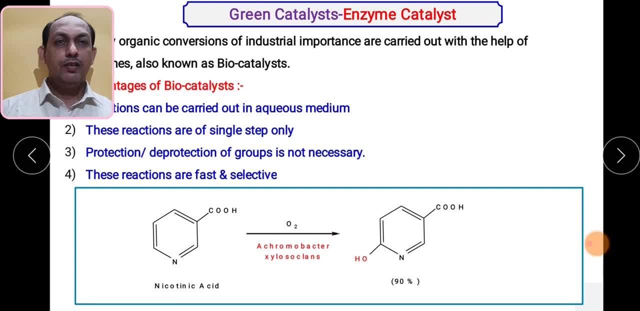 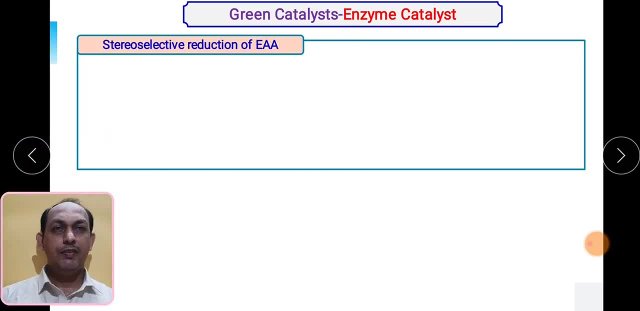 nicotinic acid hydroxylation can be selectively carried out by carrying out by a catalytic pathway. then another example is that stereoselective reduction of ethyl acetoacetate, as we know that ethyl acetoacetate is active methylene compound and it contains two carbonyl group. so this is one. 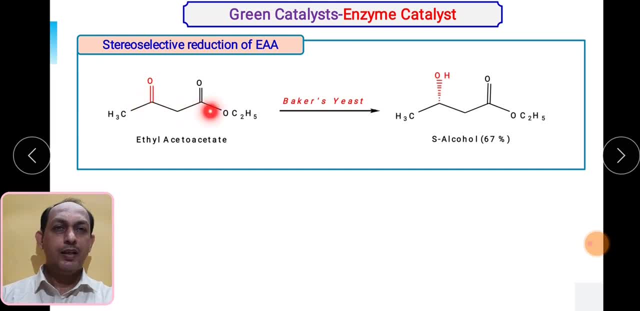 this one is ketonic carbonyl group and this one is ester carbonyl if you use the catalyst such as baker east. so there is a selective. reduction will be carried out in presence of ethyl acetoacetate takes place and the carbonyl group will get converted into COH. so you will get a selective. 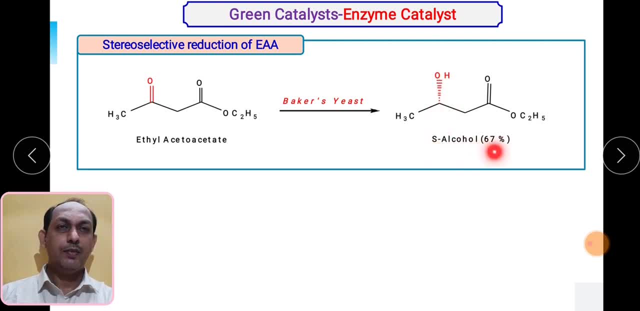 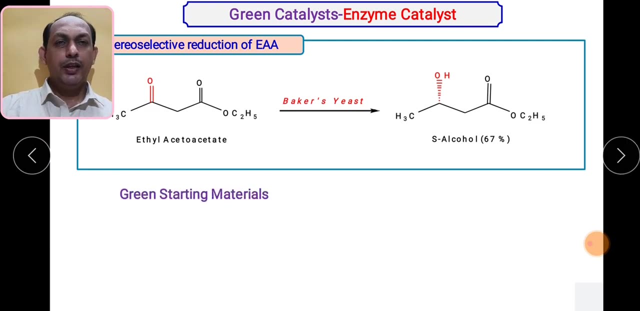 S alcohol formation with 66, 7 percent. so this can be effectively carried out by using enzyme catalyst. so these are the advantages of using green catalyst that is enzyme catalyst. so till now we have seen in the topics green synthesis we must adopt for green starting material, that starting material must be renewable and it must be very 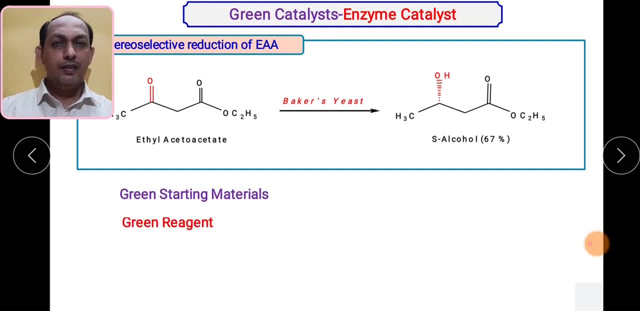 easily biodegradable inside the environment, then the reagent reagents such as dimethyl carbonate- can be effectively used as a green reagent. then the solvent is one of the important criteria which can reduce the hazardous waste formation inside the reaction. that is, green solvents. 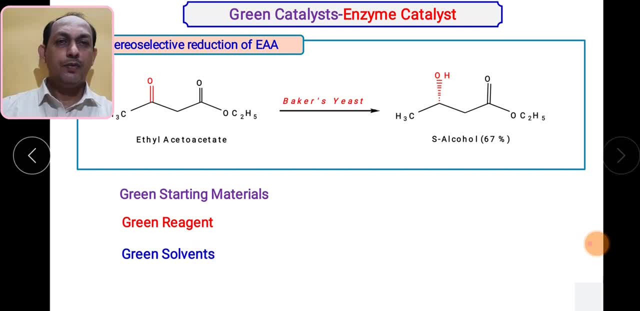 supercritical. carbon dioxide is the one of the important option for that. then green catalyst, so enzyme catalyst reactions can be very effectively carried out. so these are the four important factor which plays very important properties when we want to carry out any green synthesis. so these four things we have gone through this particular session. we have seen also various examples.